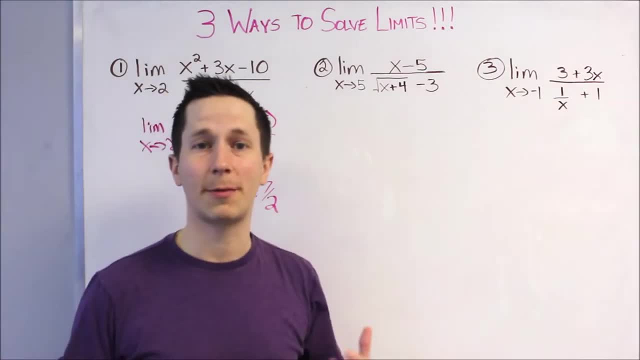 But we can't really do the same algebra here because our x is trapped under a square root. So I'm going to multiply by what's called the conjugate, which I'm going to multiply top and bottom, which you're allowed to do. 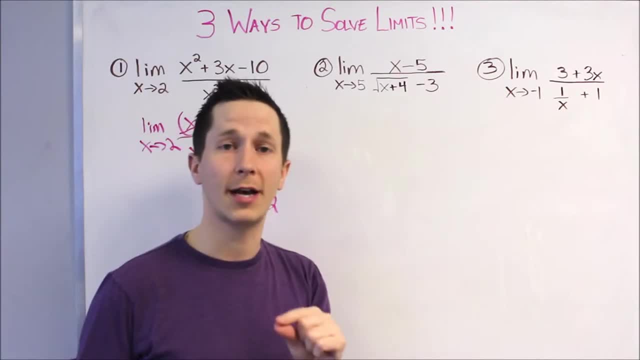 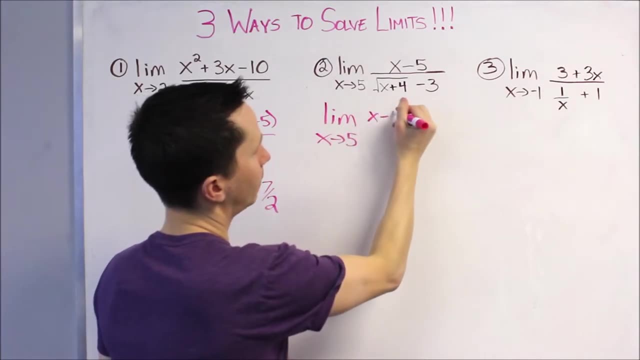 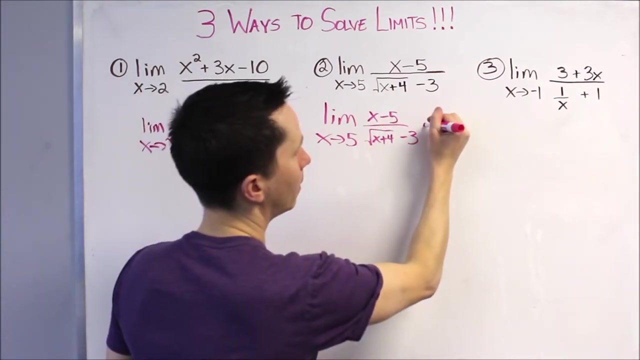 by the exact same thing that's on the bottom, except I'm going to change the sign in between, So it's going to look like this: I'm going to rewrite what we have: x goes to 5 of x minus 5 over the square root of x plus 4 minus 3, and I'm going to multiply by the square root of x plus 4 plus 3.. 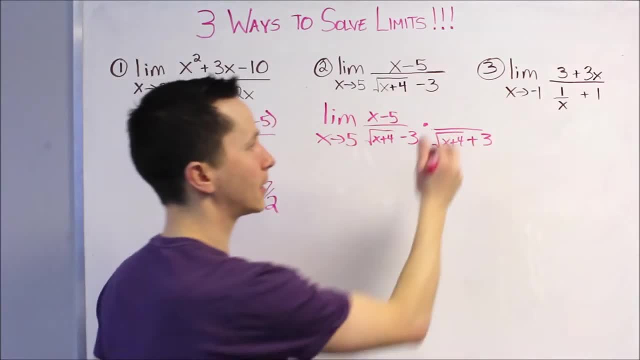 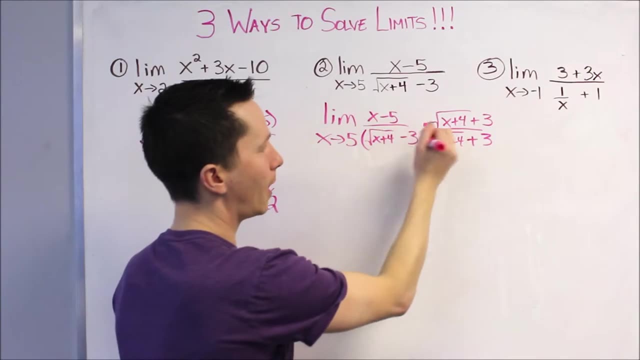 Notice: the plus is just different from the minus. Everything else is the exact same. As long as we do the same to the top, we're allowed to do it, And what that's going to do is if we look at how this bottom is going to multiply. this is a difference of squares, right. 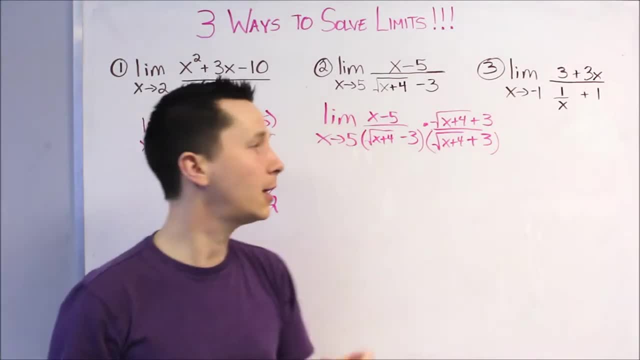 The Each bracket is the same, except for the sign change. So when you multiply it out, the middle term is going to cancel and you'll just be left with the first term squared minus the second term squared, So it's going to look like this: This is the limit as x approaches 5.. 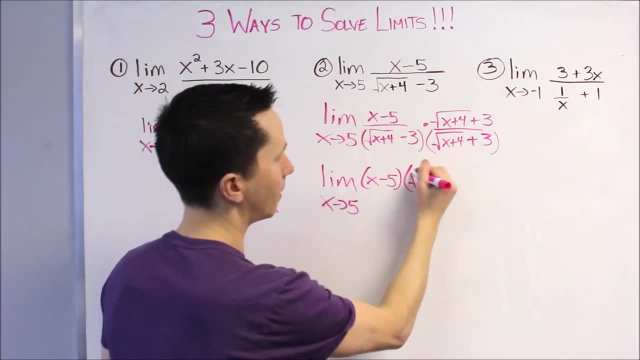 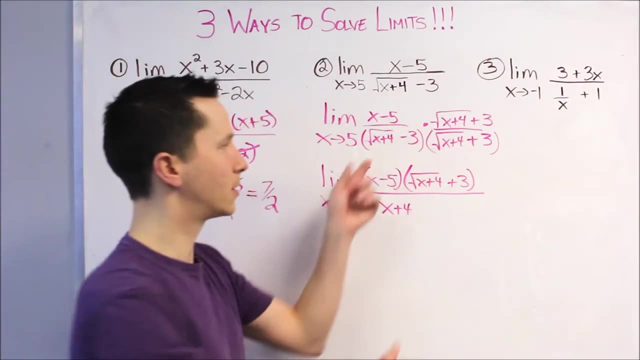 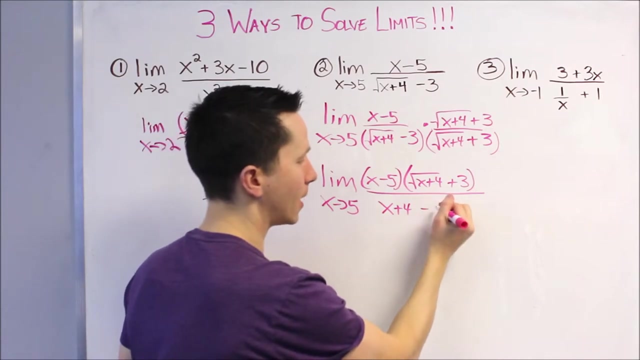 I'm not going to multiply out the top, I'm going to keep that separate. And on the bottom I'm going to get x plus 4, because the square root of x plus 4 squared is just x plus 4.. And then I'm going to get minus 3 times 3, which is minus 9.. 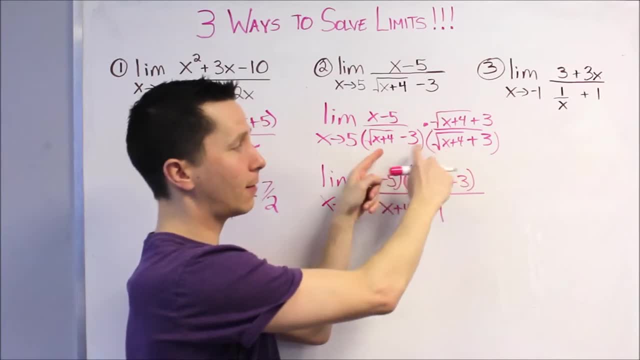 Again, if you were to do the FOIL, you'd also have an inside term of negative 3 root x plus 4 and positive 3 root x plus 4.. Those are going to cancel and that's why they're not there. 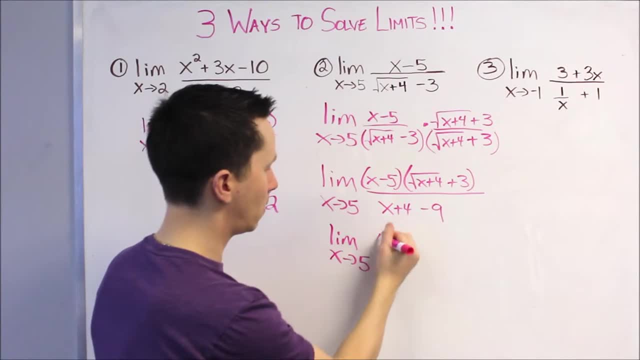 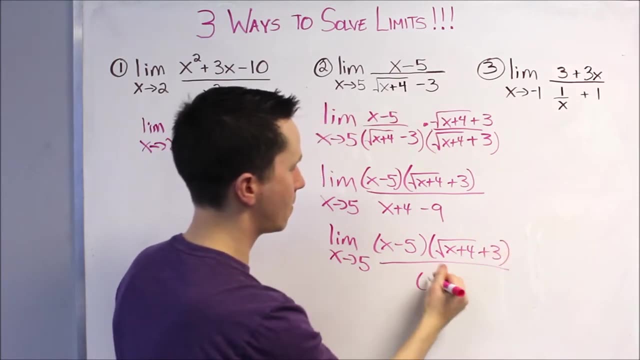 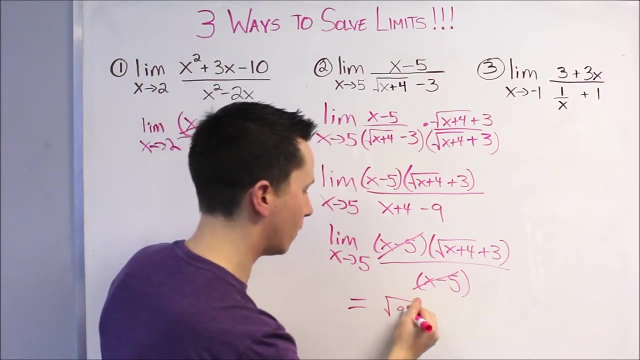 This can simplify so that the bottom is x minus 5, and then we can cancel our problem. Sub in and we get the square root of 9 plus 3, which is 6.. So the answer to that limit is 6.. 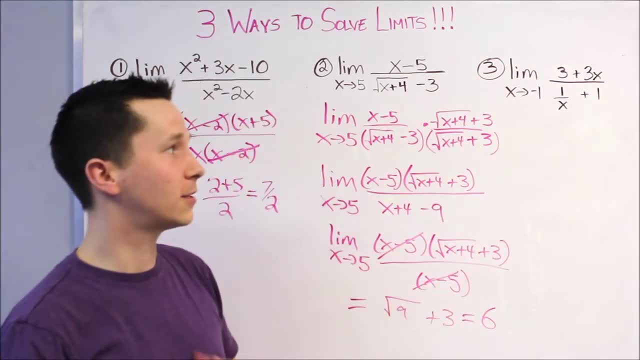 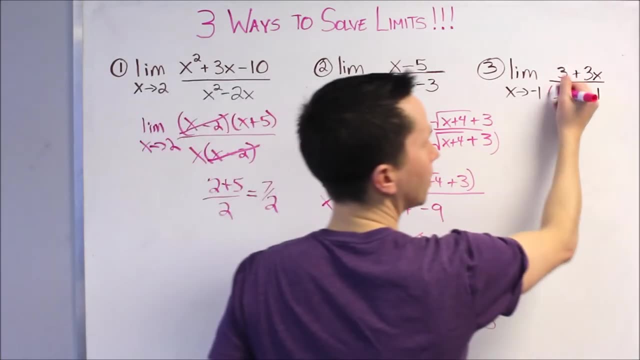 Third method, and that is where we have fractions within fractions. I'm just going to multiply everything by the common denominator of the small fraction, And that is x in this case. So I'm going to multiply everything by x, top and bottom. 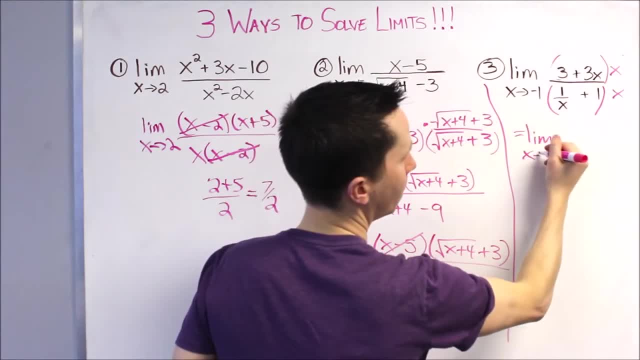 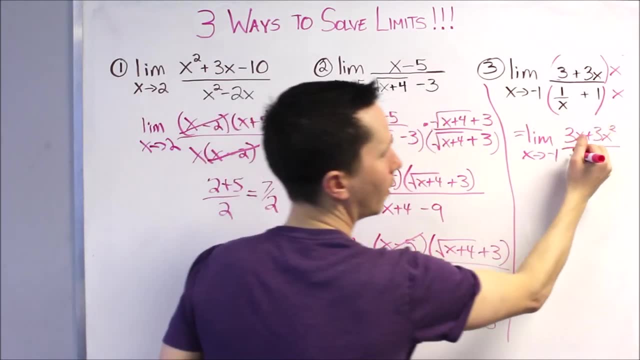 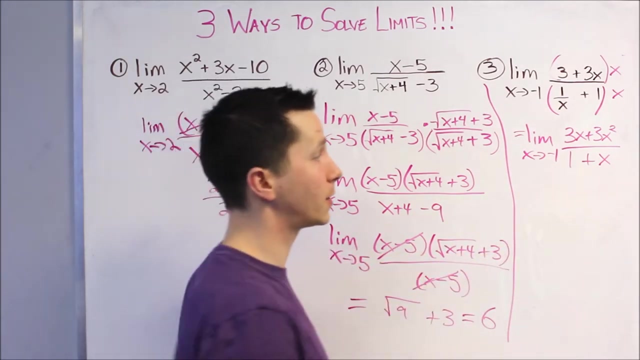 Draw a little line here. Hopefully that works out to be: We get 3x plus 3x squared on top. On the bottom x over x is just 1 plus x, And we still have an issue. If you plug in negative 1, the bottom still goes to 0.. 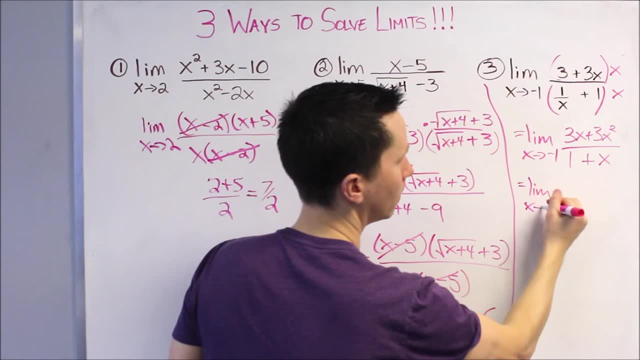 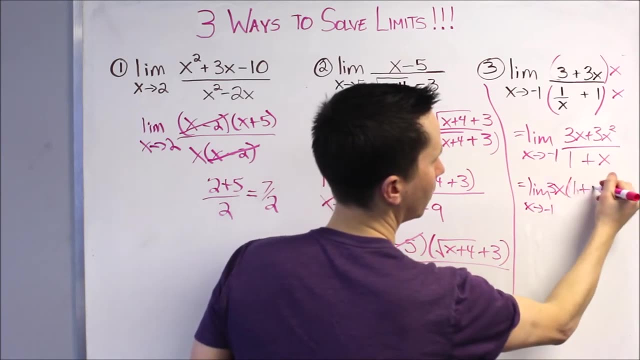 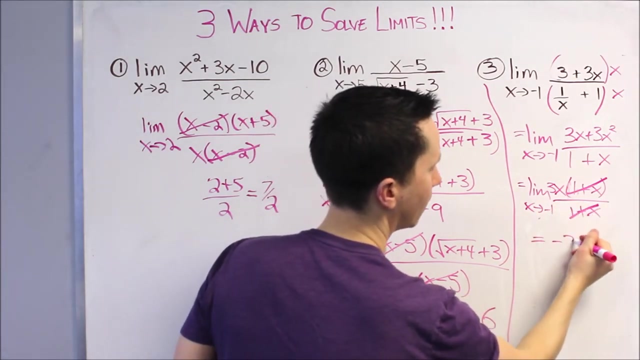 But on the top we can now factor: We can take out a 3x and we're left with 1 plus x. Now this is going to cancel our problem. Sub in now, because the problem is gone And we get negative 3.. 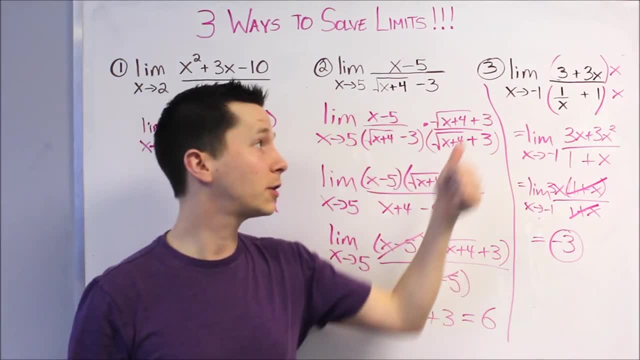 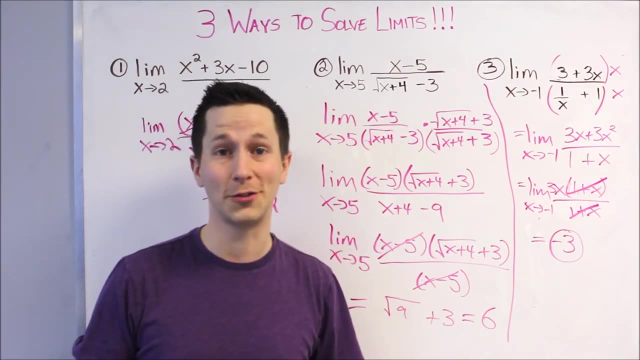 So three really solid methods: factor and cancel, multiply by the conjugate or multiply by the common denominator. Really easy way to solve limits. Thanks so much. You can always send us more questions to info at arnoldtutoringcom. 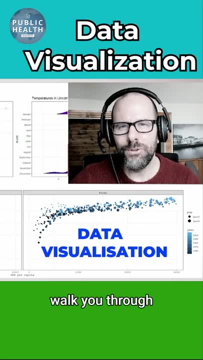 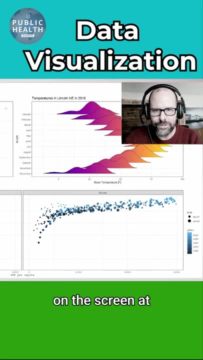 Today we are talking about data visualization, and I'm going to walk you through two things. Firstly, I'm going to walk you through the idea of telling a story with your data, and I'm going to use a couple of graphics that I've put together on the screen at the moment to teach you that. 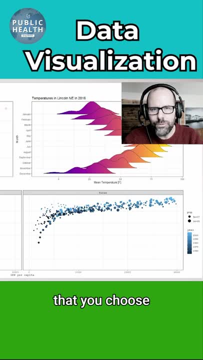 And then, secondly, I'm going to talk you through how it is that you choose between different visualization options, given the kind of data that you've got right. So exciting stuff. don't go away. stick with me, Booyahshaka. 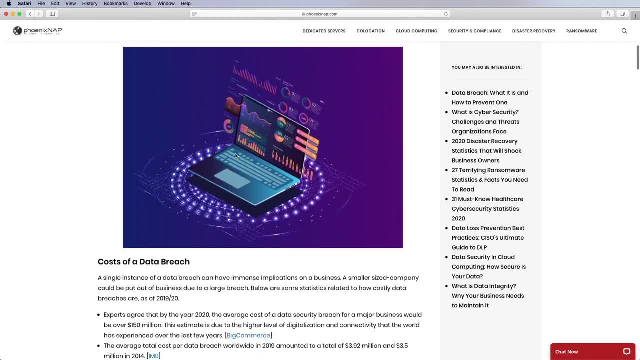 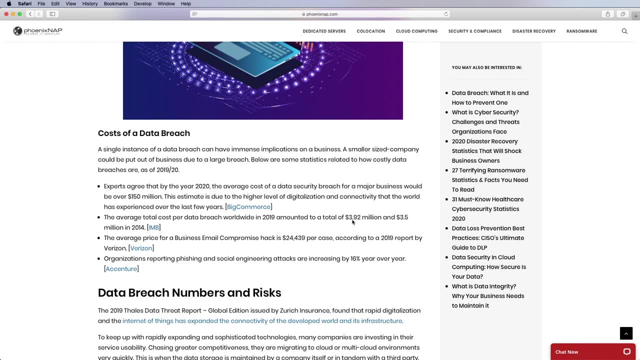 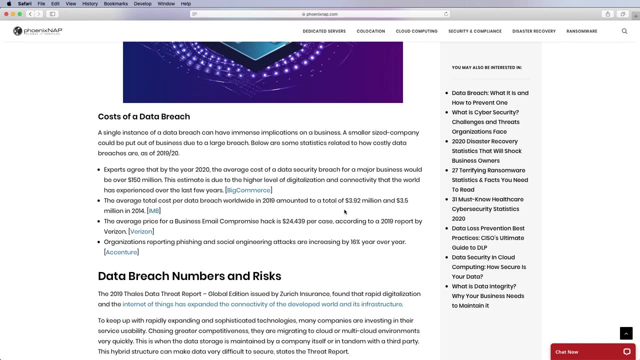 Cybersecurity and privacy breaches is a growing concern across the world today. The average cost of a breach as of 2020 was roughly 3.92 million dollars, and for a large business, would be well over 150 million dollars. There is data inherently hidden in each one of us and everything about you.